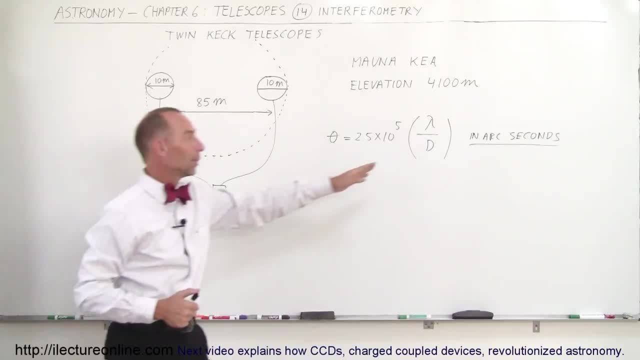 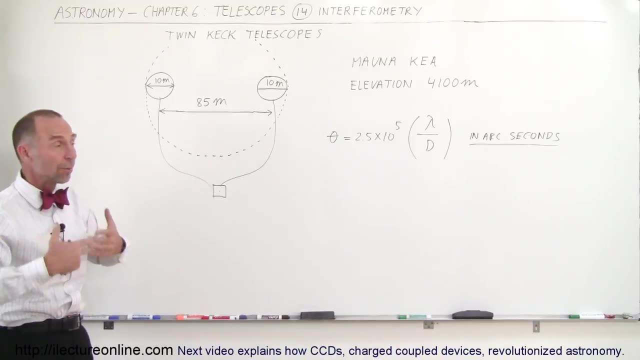 And by doing that we actually increase the resolution and we can then put 85 down there instead of 10, and have even a smaller angle of resolution. And then, if we use adaptive optics to make sure that the images are clear so we don't have to worry too much about the turbulence of the atmosphere, we get very high resolution images. 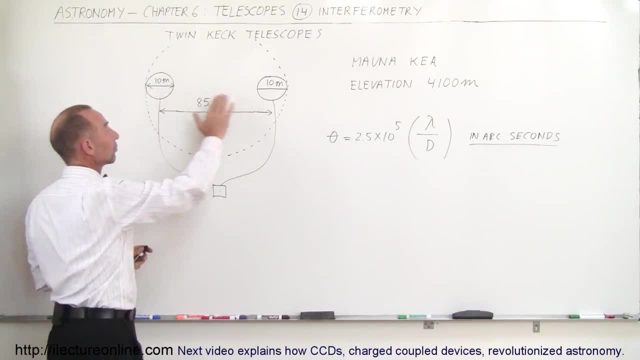 The only drawback is you still only have these collecting areas for the picture, so the area is still pi? r squared and the diameter being 10 meters, meaning a radius of 5 meters. So the total surface area of these two are only 10 meters. 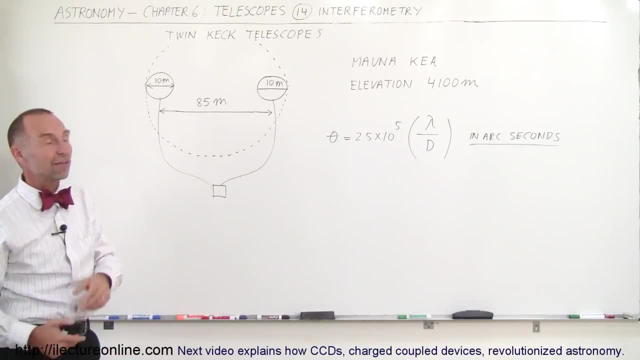 So we have only twice pi r squared, or twice pi times 5 meters squared- Still quite an accomplishment. So the idea is, even though we don't have the large collecting areas as if it was one giant telescope, we still get the resolution angle, which is what we're after. 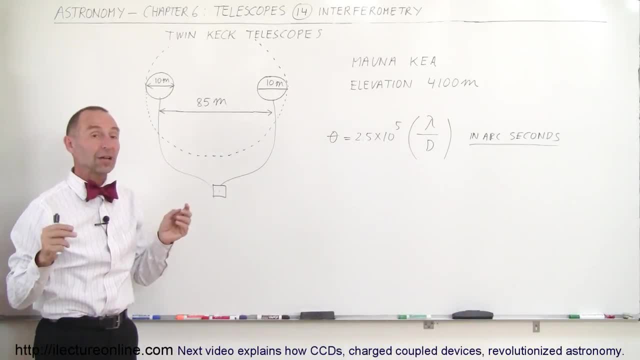 Very, very high resolution angle. In some cases we actually have computers that work on different continents at the same time looking at the same image, linked via computer and the internet processing the images together to have very high resolution. We use that usually for radio telescopes, but we could also use it for visual telescopes. 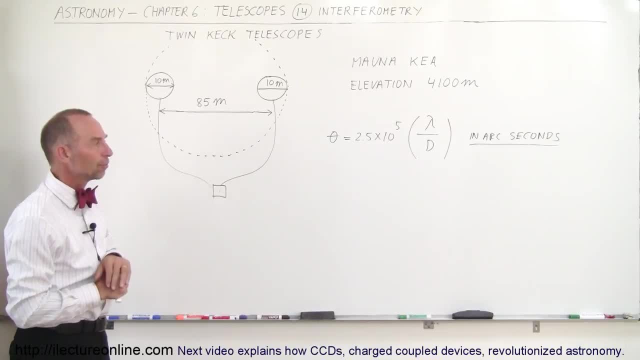 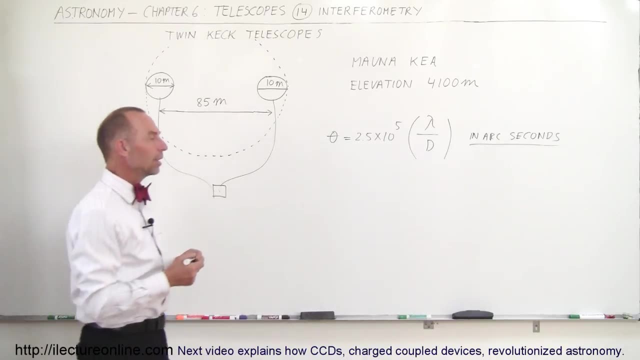 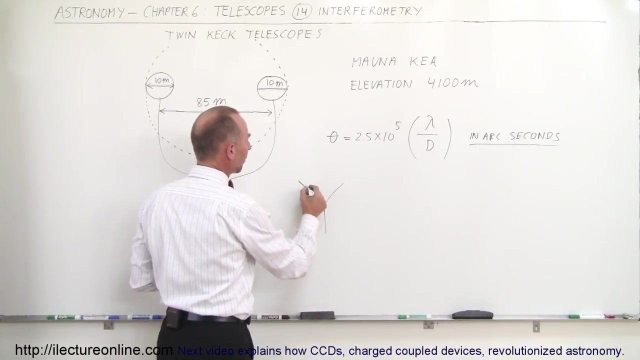 Again, it's all about sharpness of the image and the angle of resolution. So that's one way- interferometry, in which we can take care of that. Radio telescopes have a tremendous ability. We can actually put these large radio telescope antennas on, for example, railroad tracks, where we put antennas spaced apart like that and we can move them back and forth in such a way that we actually have a relative diameter. 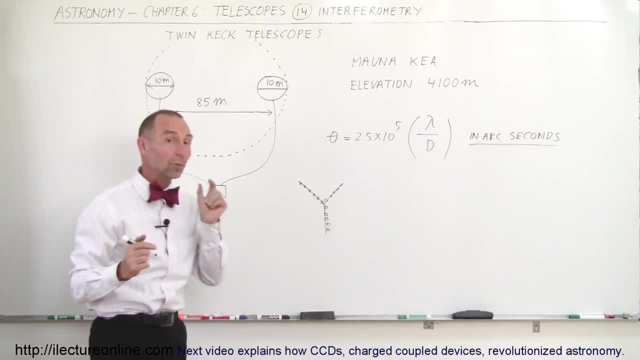 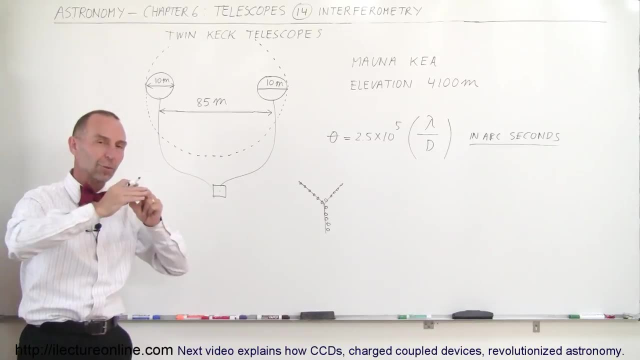 That is equal to this distance right there. Otherwise radio telescopes have very poor resolution. but by building a system like that we have multiple radio telescopes spaced apart like that in different directions. We can kind of mimic one giant radio telescope. 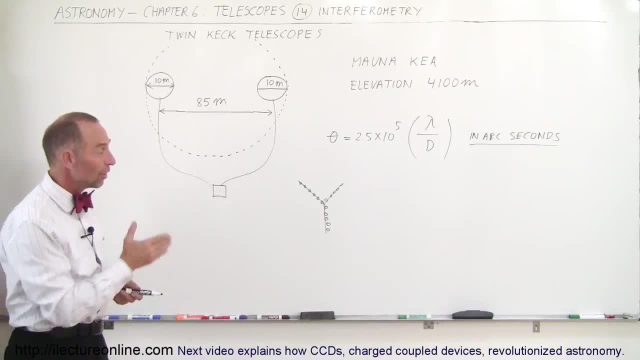 So interferometry is one of these great techniques that we use to get the best resolution out of the equipment that we have.